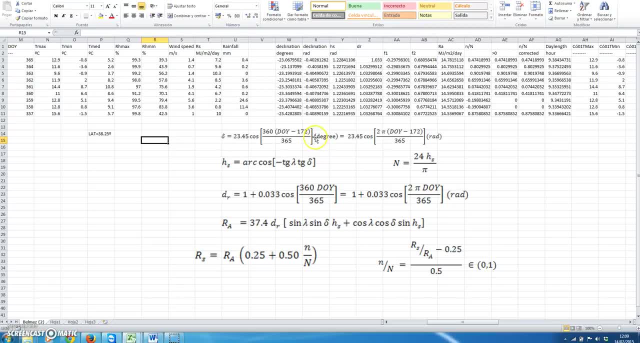 The equation for calculating solar declination is the one appearing here. If we use a pocket calculator, the sine cosine functions will use angles in degrees. If we are using Excel, as in this case, we need to use the angles in radians. 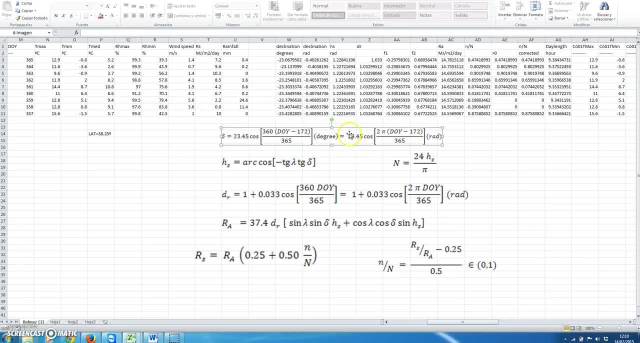 In this case, the equation would be like this: 23.45 pi cosine of 2 pi day of year minus 172 over 365.. That's the equation that we will put for this cell: 23.45 pi cosine of 2 pi day of year minus 172 over 365. 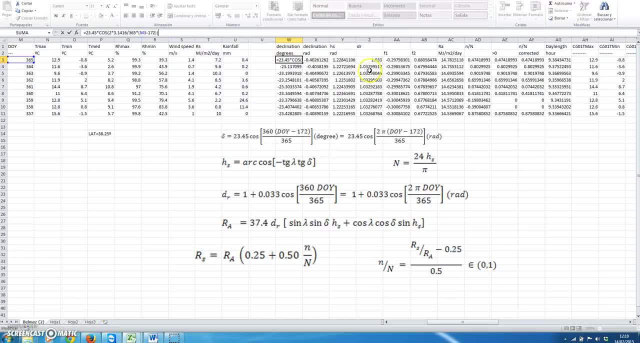 That's the equation that we will put for this cell: 23.45 pi cosine of 2 pi day of year minus 172 over 365.. And we would get this data that appears here in this column. That provides the declination in degrees. 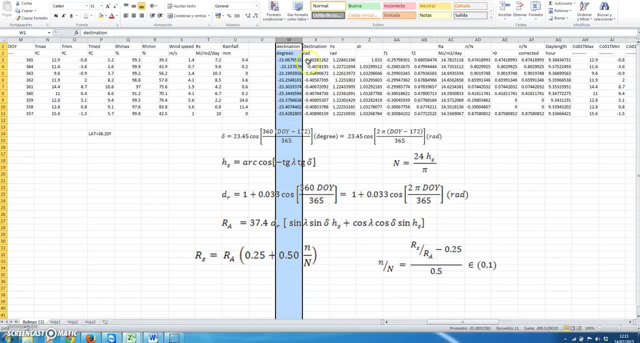 Then we convert the declination in degrees to rad. How we do that? But simply by multiplying by pi and then dividing by 180.. Ok, So now in this column we have the values of solar declination in radians. Next we're going to calculate a variable called hs. 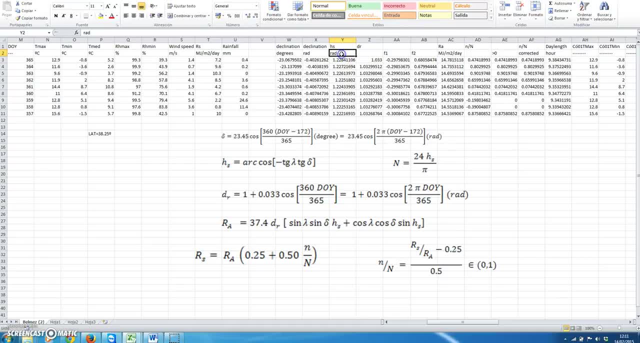 which is half of the day length expressed in radians. To do that, we apply this equation. Apply this equation. This is the r cosine of minus Of minus the tangent of the latitude. See that the latitude is now expressed in radians. We need to do that always when we are working with Excel. 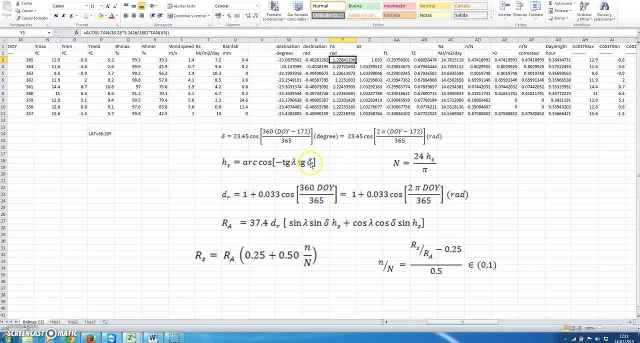 Multiply by the tangent of the solar declination, which was the previous column. Now that we have the variable hs, we could go and directly calculate the day length, which is this column, applying this equation, Multiplying hs by 24 and dividing by pi. 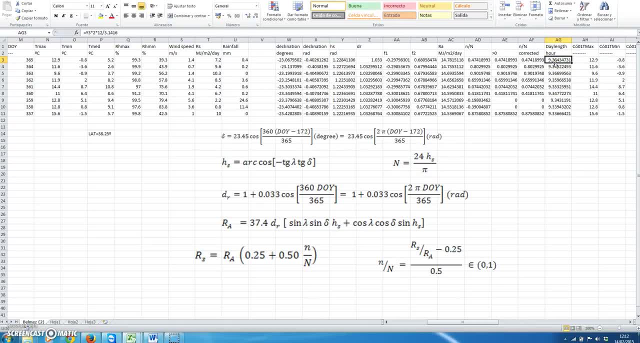 we get the day length in hours. We see that in December in Vermont we have day lengths around 9 hours. Ok, Next we calculate a variable which corrects solar radiation data for the distance from the Earth to the Sun. This is the variable d sub r. 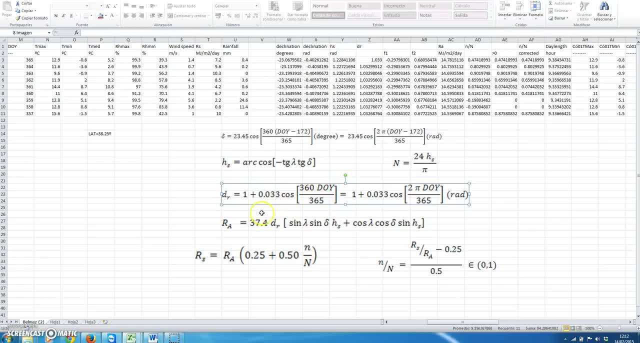 If we used a calculator, we would apply this equation, but as we are using RAN, we apply this equation. Ok, Then we calculate the r by putting here the equation for operating with radians. Then we apply the equation for extraterrestrial radiation. 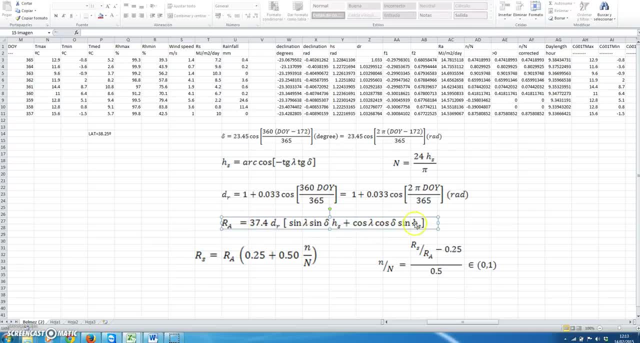 r sub a, which is this one. I have just divided the calculation in two steps. First I calculate this triple product. I call it F1. And it is the product of the sign of the latitude. Look that the latitude is in radians. 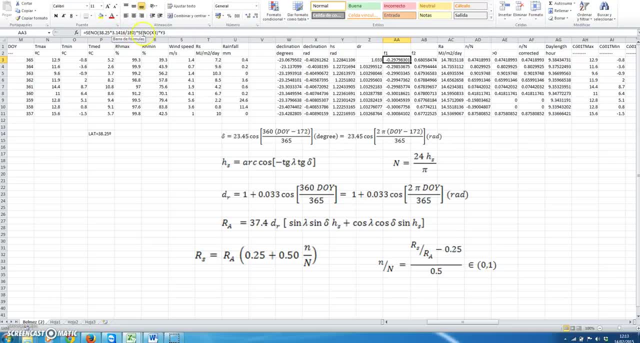 Multiplying by pi divided by 180.. Multiplying by the sign of the declination And then multiply by the value of hs. The second term in this equation is cosine of the latitude, cosine of declination and sine of hs. That's the one up here. 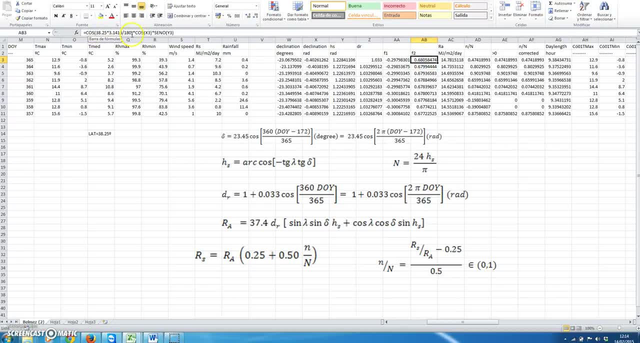 Cosine of the latitude in radians, cosine of the declination and sine of hs. Ok, And then we can multiply to get rA. We just multiply 37.4.. Multiply by dr, Same here, Plus the sum of the previous two columns. 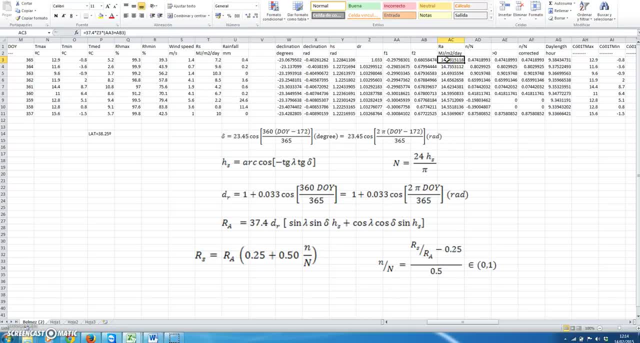 Then we get the extraterrestrial radiation. In this case it's around 15 megajoules per square meter per day. This would be the total solar radiation that would reach this location on that given day if there was no atmosphere. On the average, 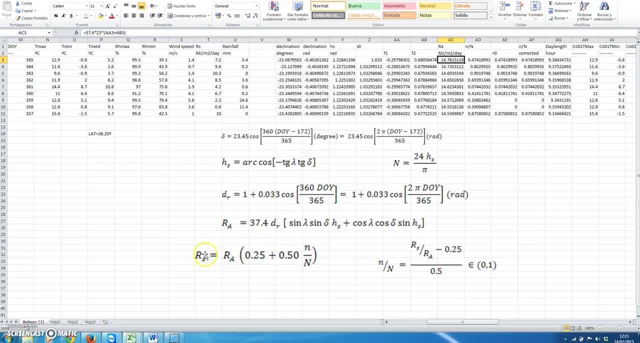 the solar radiation reaching any place on the Earth can be calculated using that extraterrestrial radiation and taking into account the degree of clear sky. The degree of clear sky is the quotient between the actual duration of clear sky over the maximum number of hours of clear sky. 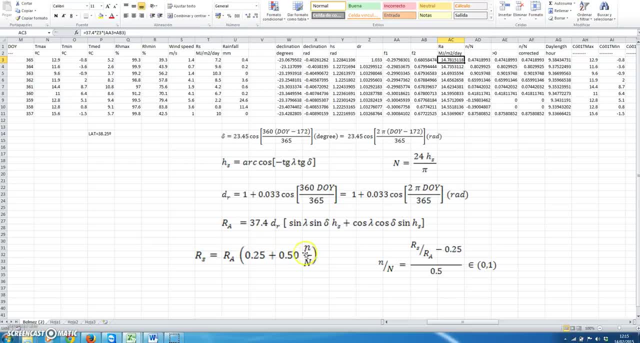 which is exactly equal to the day length. We don't need to apply this equation In this case, because we have measured solar radiation in this water station. is this column Ok? But as we have this equation, we can deduce the fraction. 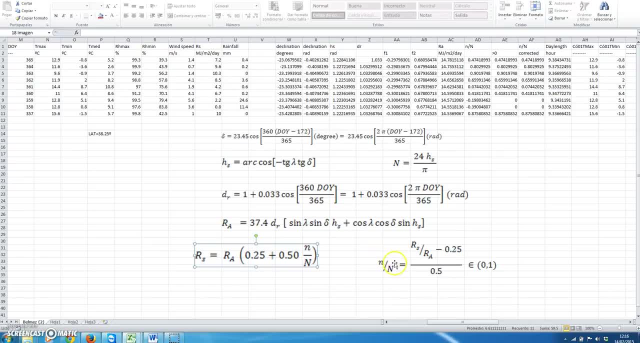 or the degree of clear sky using the measured solar radiation, the calculated extraterrestrial radiation and these two coefficients. Note that if the sky is completely overcast, the fraction of clear sky would be zero and, in the best, in the maximum case. 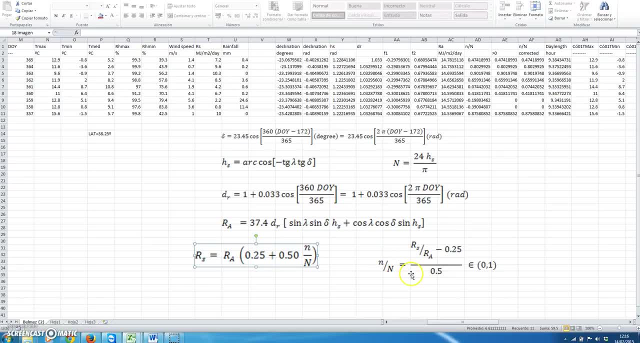 the fraction of clear sky would be one when the sky is clear throughout the day. Now, applying this equation, we can calculate here the degree of clear sky using this equation and we have these values, As we know that these values have to lie between zero and one.